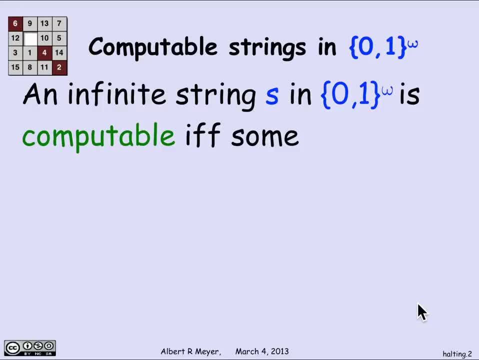 uncountable number of infinite binary strings, And that's because there was a simple bijection between the infinite binary strings and the subsets of the natural numbers, That is, the power set of n. Let's look at the strings in the infinite binary string. 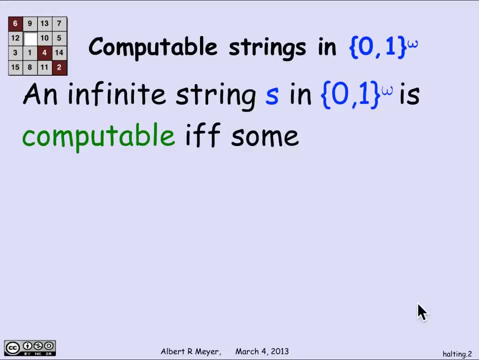 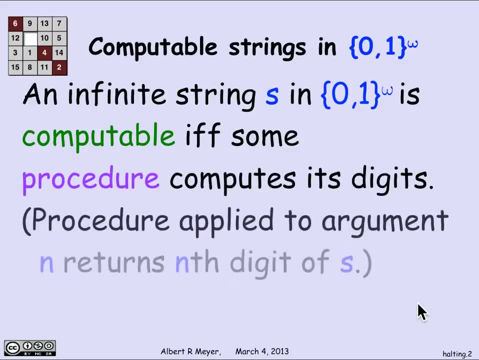 So what I mean by a computable string is that there's simply a procedure that will tell me what its digits are. So what I mean is that the procedure applied to argument n will return the nth digit of the string, s. That's the definition of what I mean by saying s. 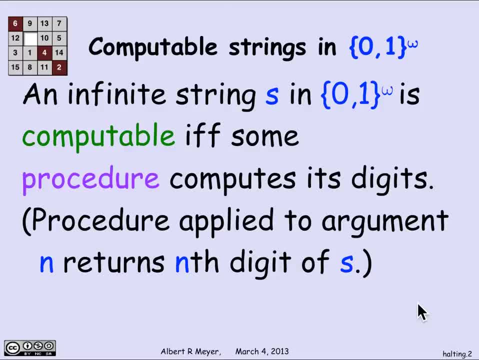 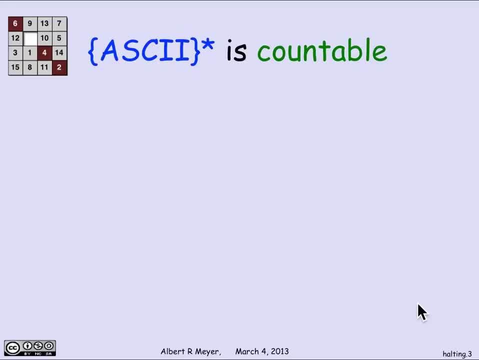 is computable. I can compute its digits, whichever digits are needed. Now we saw that there were only a countable number of finite binary sequences, And I mentioned that now because I want to think about sequences over the slightly larger alphabet, instead of 0,, 1, the 256 ASCII characters And, by the same argument, the set of finite ASCII. 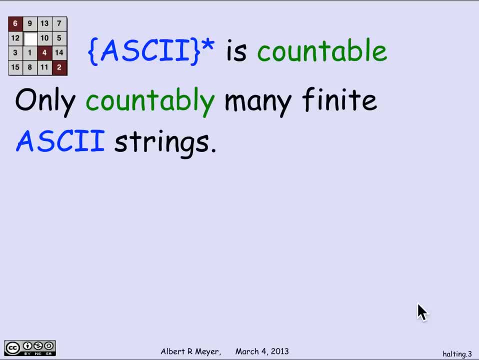 strings is also countable. You just list them in order of length, the same argument that we use for the binary strings. Now, the point of looking at the ASCII strings, the 256 keyboard characters, is that every procedure that we enter into argument n will always be limited to a set of finite binary. 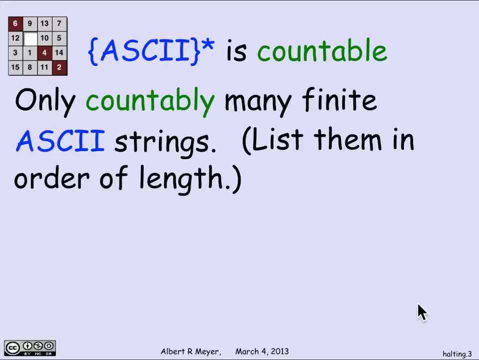 strings a computer. we type in an ASCII string. Every procedure can be represented by an ASCII string And since there are only countably many finite ASCII strings, it follows that there are only countably many computable procedures. 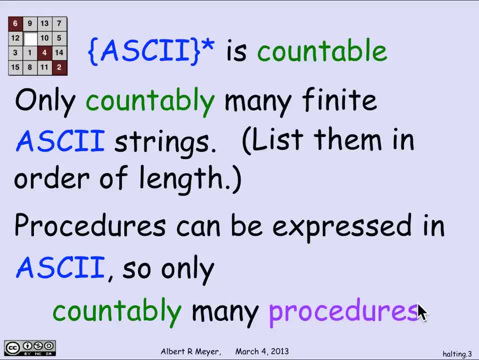 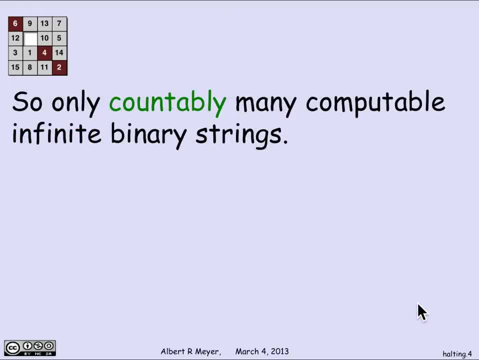 Now, since, in order to be a computable infinite binary string, there has to be a procedure which computes its digits, we can immediately conclude that there are only countably many infinite binary sequences that are computable, only countably many computable infinite binary sequences. 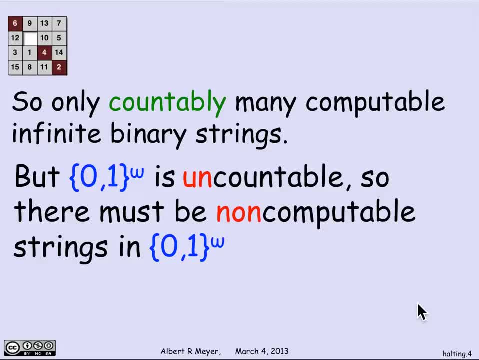 But I already said, there are an uncountable number of those infinite binary sequences. so it has to be that there are non-computable sequences, non-computable infinite binary strings that exist. So we can conclude that, as a matter of fact, 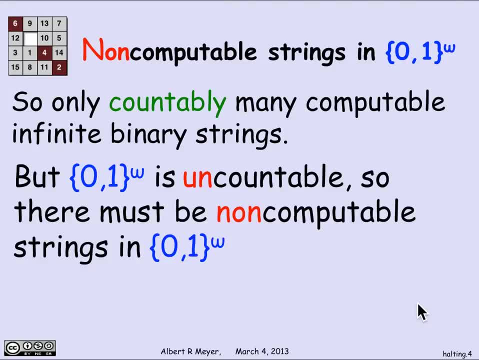 since the set of infinite binary strings is uncountable and the computable ones are a countable subset, there have to be an uncountable number of non-computable infinite binary sequences. Most infinite binary sequences are actually not computable. 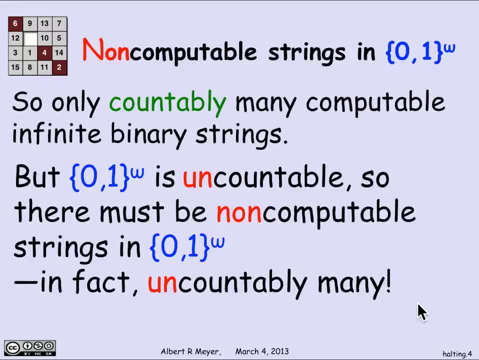 OK, that's kind of abstract thing to know. They're out there and you can't get a hold of them computationally. but the reasonable question to ask is: what do they look like? And what we're going to see is that, if you consider 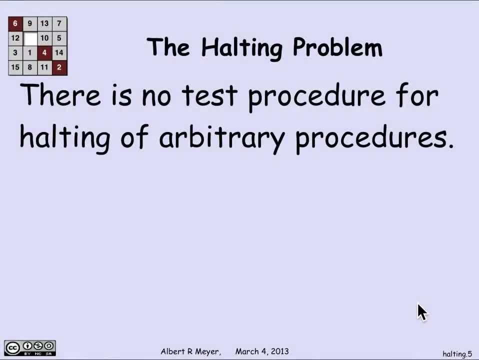 a particular, a sensible, concrete computational problem of giving a procedure, figuring out whether it will run and return a value successfully on some argument or not is called testing the halting property of procedures. I want to know, given a procedure and an argument, 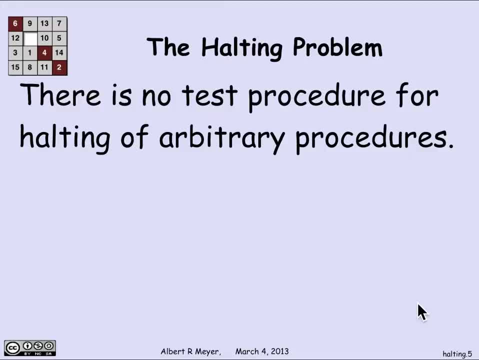 that I could apply it to. does it return a value or does something else bad happen? It runs forever. It returns an error, We don't get a satisfactory value out, And if it does satisfactorily return something, we say it halts. 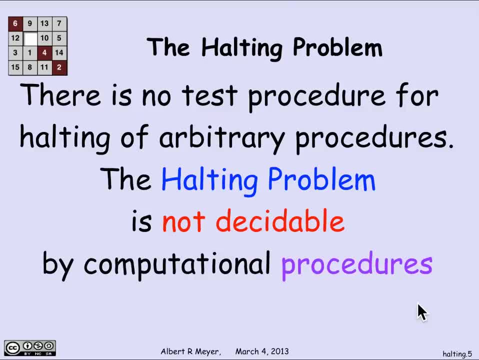 And what I'm going to argue is that the halting problem is not decidable, That is, there's no procedure which, given an input that describes a procedure, the fixed procedure can figure out what its input is doing. Let's look at that in more detail. 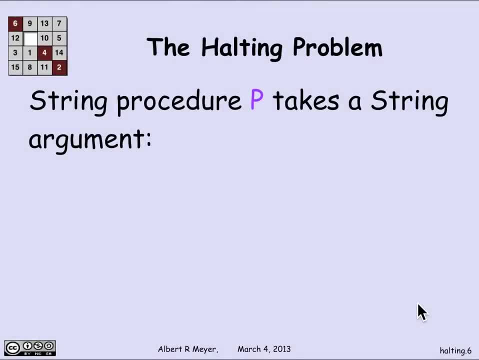 So let's think about string procedures, because we're thinking about procedures being represented by ASCII strings. So let's think about procedures that take a string argument. So an example of a procedure P: it might be that when you apply P to the string no, it returns 2.. 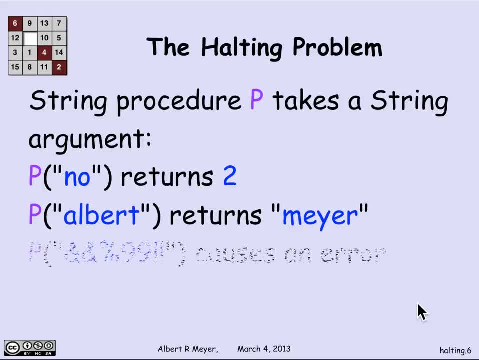 When you apply it to the string Albert, it returns Meyer. When you apply it to this string of weird symbols, that causes an error. And you apply it to the sequence of characters, what now? and it actually runs forever. These are just illustrations of the kind of behavior 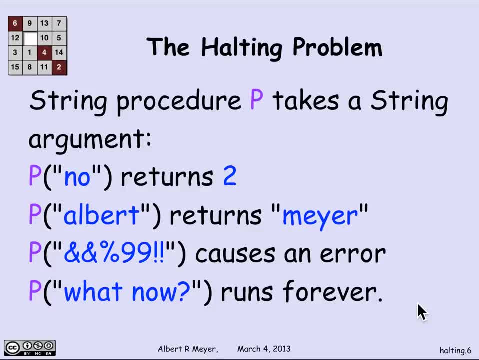 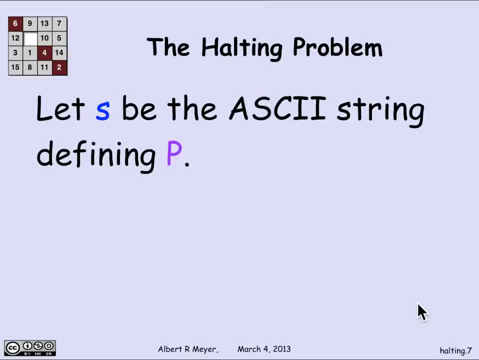 that some weird string procedure might exhibit. So what I want to think about is: suppose that I have an ASCII string X, a finite ASCII string- that's the one that defines this procedure- P When I'm trying to run P on the computer. 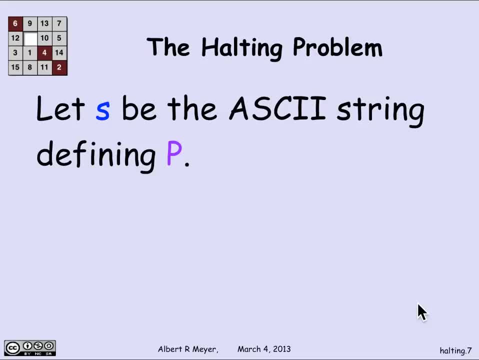 I have to type in S in order to give the computer the definition of P, to tell it what to do, And I'm going to say that S halts. The string has this property called halting or halts If, and only if, this procedure P that S describes. 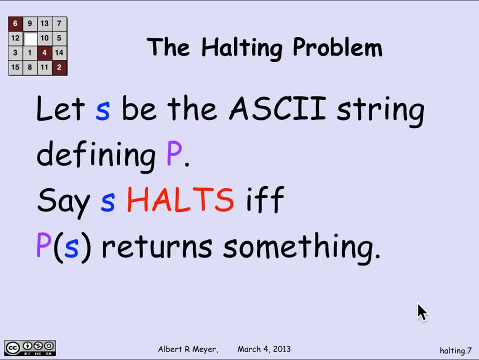 returns successfully when it's applied to S. This is where we're really doing a diagonal argument. We're taking the S object, the procedure that's described by S, and applying it to S, And that's kind of going down the diagonal of S applied to S or the nth element. 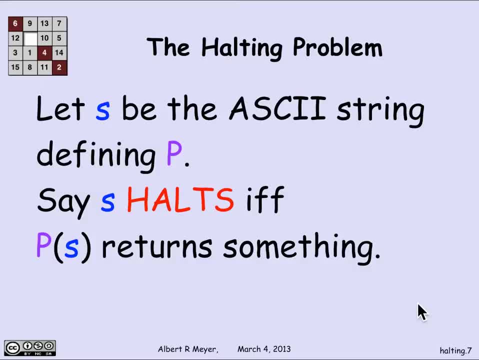 of the nth row in the pictorial diagonal argument. That's the idea that we're going here. But let's just go back to the definition. A string is set to halt if, when you interpret it as the description of a procedure that takes a string. 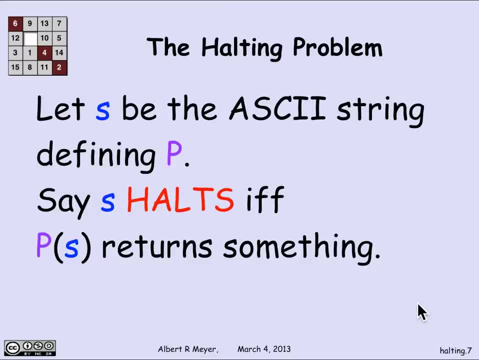 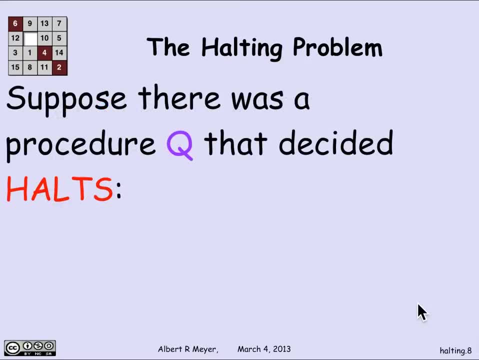 argument, You apply that string procedure to that very same thing S you successfully return. That's the halting problem, And what I want to argue is that it's impossible that there could be a procedure Q that decided the property halts of strings. 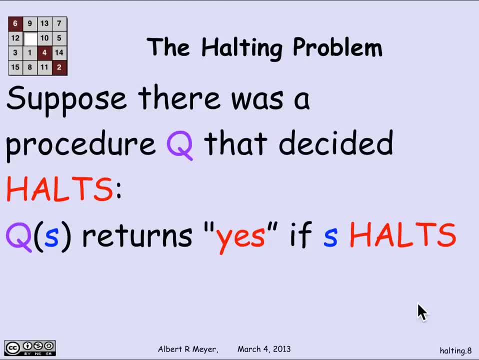 That is to say, Q applied to a string returns yes if S does return successfully. if S halts And it returns no. otherwise Q applied to S will say no If S runs forever or if S has a type error. 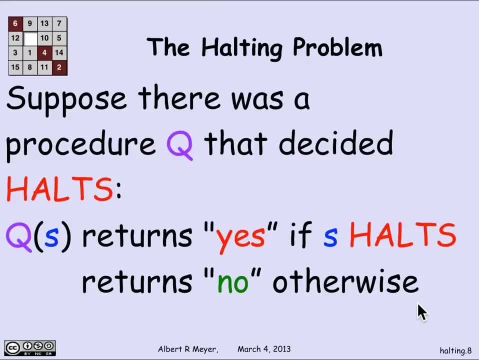 or S does anything other than successfully return a value. Let's suppose, for the sake of contradiction, that there was this: halts desire. I claim there can't be such a Q. for the sake of contribution of contradiction, Let's assume there was one. 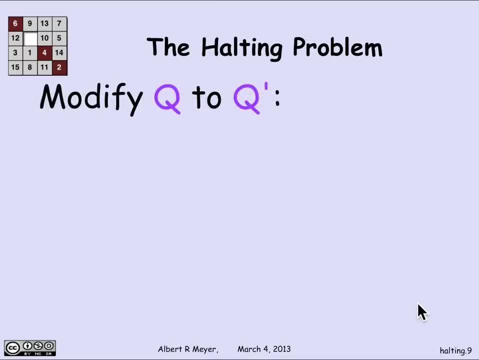 Then this is the trick that I'm going to do: I'm going to modify Q to act as though it was complementing the diagonal More precisely. This is what I'm going to do: I'm going to modify Q to be another procedure: Q prime. 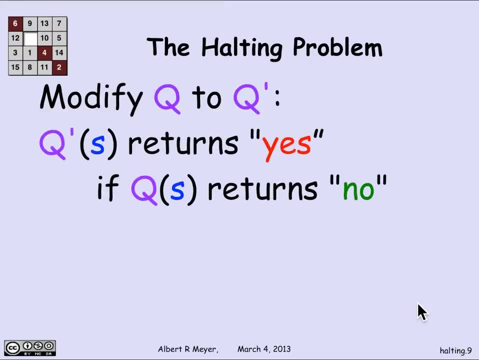 which just behaves a little bit differently, Namely Q prime of S returns yes when Q of S returns no And Q prime of S returns nothing, That is, it doesn't halt if Q of S returns yes. So Q prime is like complementing the bits on the diagonal. 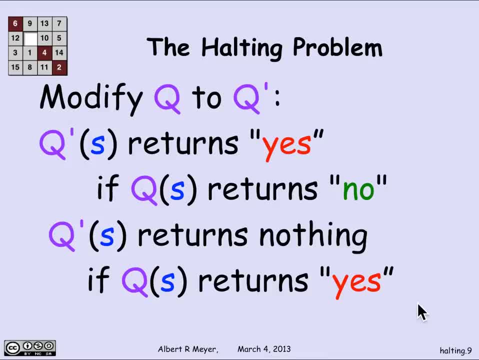 But here's the precise definition: Q of S says no, Q prime of S says yes, Q of S says yes. Yes, S halts successfully. Q prime then does not halt successfully, It returns nothing at all. Let's go crank through the consequences. 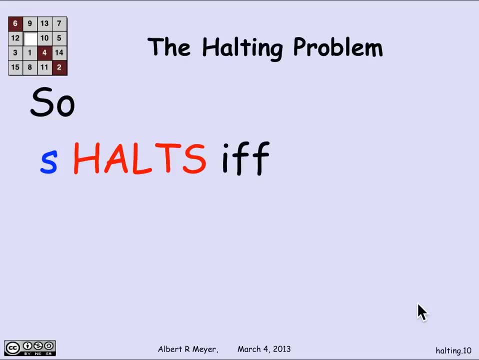 of these definitions. So S halts means Q prime of S returns nothing. That was the way we defined Q prime of S. Now let's let T be the text for Q prime. We said that Q prime was a if Q is a procedure. 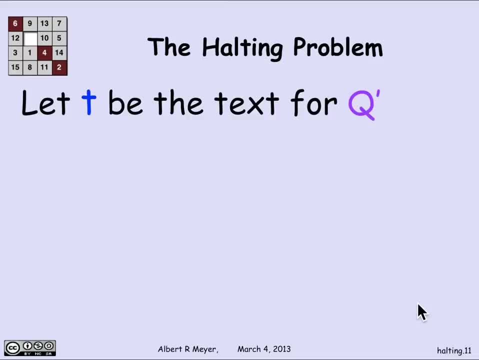 then surely we can tweak this procedure Q to get the procedure Q prime. So Q prime will have a text that describes it. It'll be the ASCII string that defines Q prime. Let's let T be that ASCII string. What do we have? 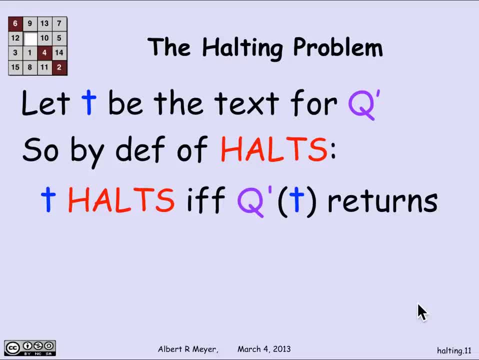 Then, by definition of halts, T halts if and only if the procedure that T describes, namely Q prime, applied to T returns a value successfully. Now, by definition of Q prime. however, Q prime was the thing that on T. It returned a value successfully if and only. 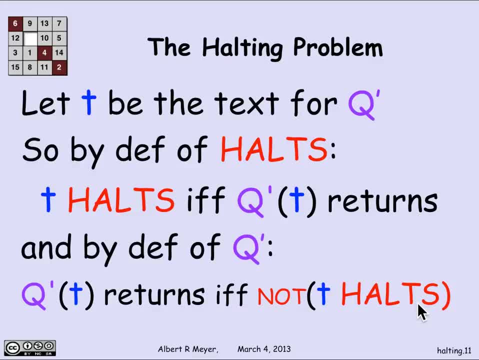 if it was not the case that T halts. So if you put those two things together, that is, we're looking at T halts if, and only if, Q prime of T returns and Q prime of T returns a value successfully, if, and only if not T halts, then put the two together. 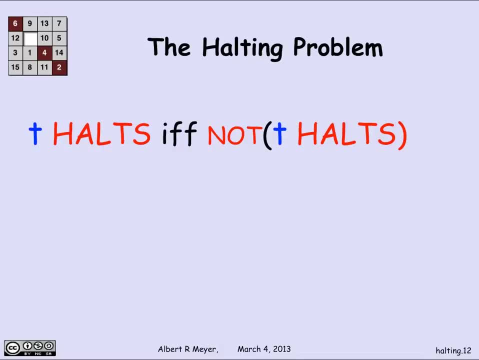 and we have a contradiction: T halts if, and only if, T doesn't halt. And that contradiction says that our original hyperbolic hypothesis that we had a Q that would decide the halting problem, can't be right. It's impossible to write a procedure that. 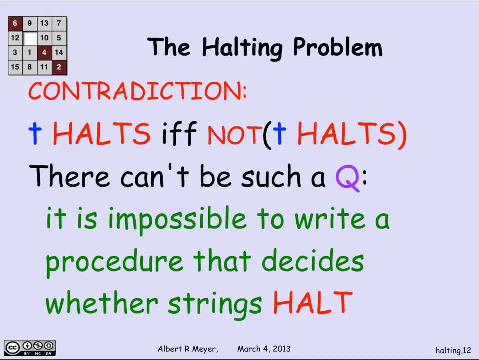 determines of strings whether they describe a procedure that halts when applied to itself. That at least gives us some concrete problem that we can say is not something that a computer can do. Even though it's a very well-defined and clear question, it's just not possible to get. 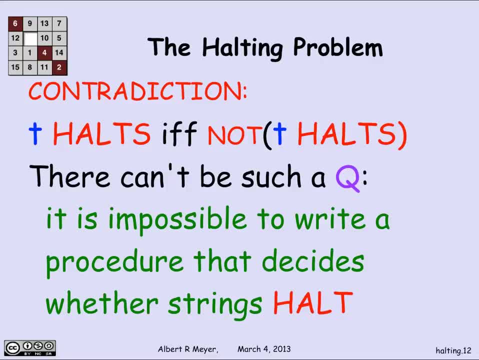 a computing procedure that will, on an arbitrary string, figure out the right answer. Any program that applied to strings is trying to do this job. Either it will give the wrong answer or, if it never gives a wrong answer, it means it doesn't give an answer at all on some strings. 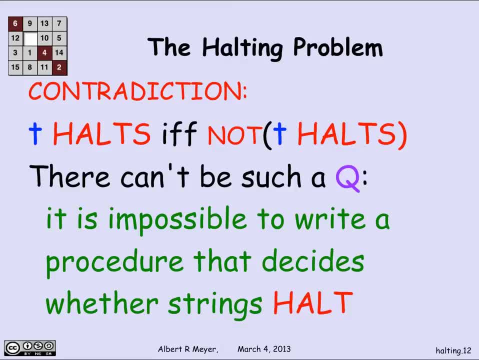 All right. Well, you could say that I don't really care very much about whether a program halts or not. So let's look at: how do you apply the same reasoning? or, more precisely, how do you apply the same reasoning? OK, 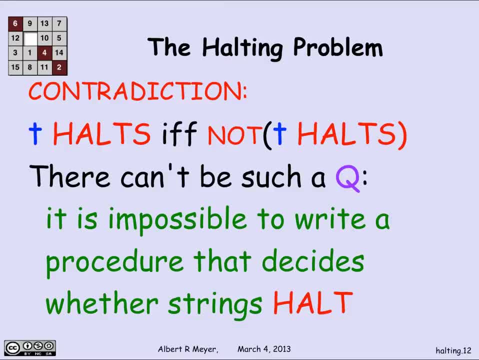 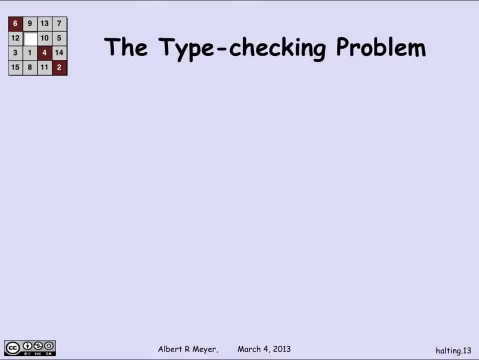 Let's look at how do you apply as a corollary of the fact that the halting problem is not computable, Let's talk about something that sounds closer to a practical interest, namely type checking. So I want to think about the type checking problem. 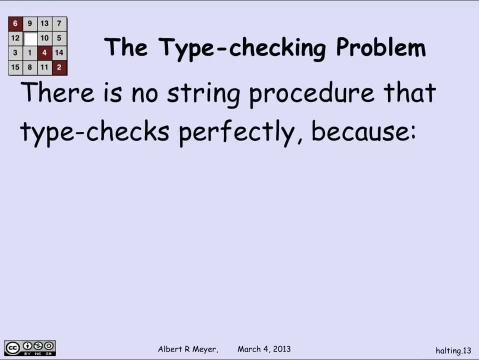 And what I want to say is that, in fact, there's no string procedure that type checks procedures perfectly, And so what I mean is that I want to be able to write a program that will look at a program and test an ASCII string that describes a procedure. 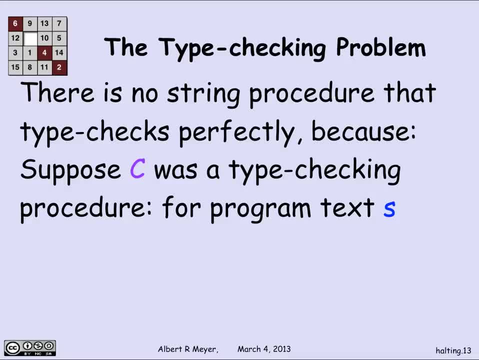 and figure out whether that ASCII string, if you ran it, would cause a runtime type error. That's what type checkers are supposed to do. They're supposed to check your program, figure out whether the program will cause a runtime type error. 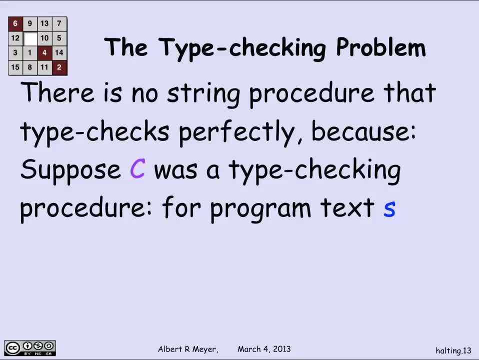 If so, it reports it. If not, it says this program is safe. Other things may go wrong, but it's not going to commit a runtime type error. So let's suppose that I had- OK, I had- such a type checking procedure C. 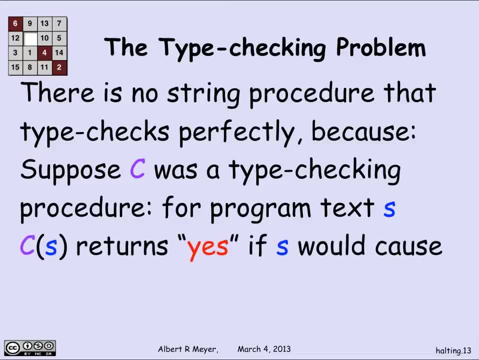 So what that means is that for program text S: C of S returns yes if running S would cause a runtime type error and C of S returns no, the output string: no otherwise, if S would not cause a runtime type error. In other words, S is safe. 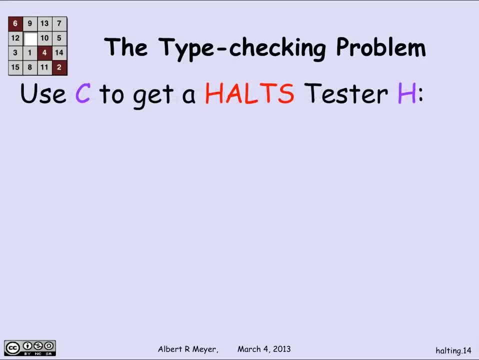 All right. Now what I claim is that if you give me C, if I have a procedure, that's this perfect type checker, I can use C to build a tester for holts, which we said is impossible. So how would I use C to get a holts tester? H? 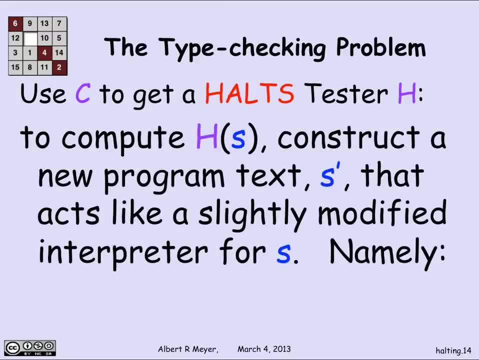 Here's how I'm going to tell you how to compute H of S. I'm going to write a procedure. I'm describing the procedure that this tester H carries out on argument S And what it does is: given argument S, it's going to construct a new program. that's a small modification. 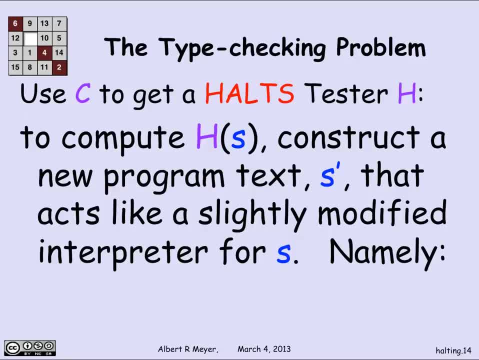 of S. It's going to construct this new program, S prime. that acts like an interpreter for S. So S is a computer program or procedure. I want to know whether, if you just run it, it'll halt or not. I'm going to tweak it a little bit. 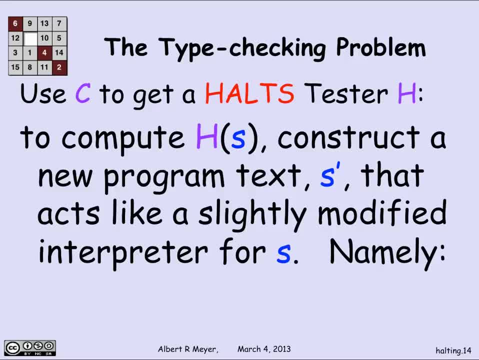 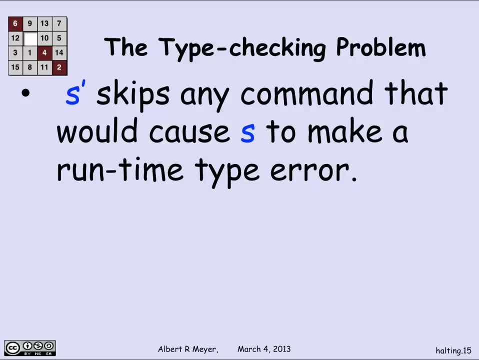 so that S prime acts like S, but in a slightly modified way. And here's how S prime works. S prime is going to be an interpreter that's simulating step by step how S behaves, But at the moment that it discovers that S is about to commit a runtime type error, 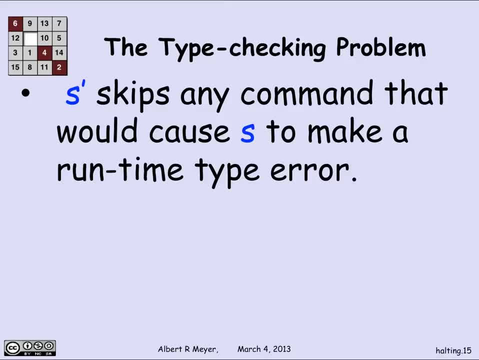 that the next instruction that S prime would execute in simulating S was going to be a runtime type error, S prime would just skip it And who knows what the consequences of skipping it will be. but it'll skip it and just keep going. 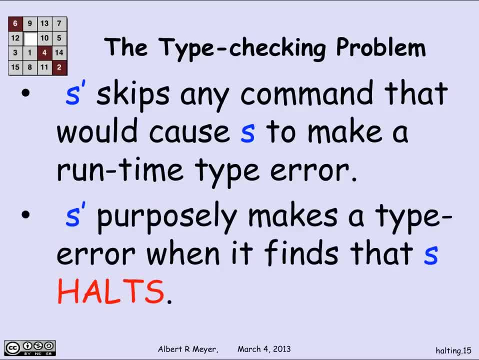 OK, And if S prime, in simulating program S, discovers that In fact S returns successfully, that is, S halts, then S prime will purposely make a type error. So let's think about what that means. Well, actually, let me just wrap up what the definition of H is. 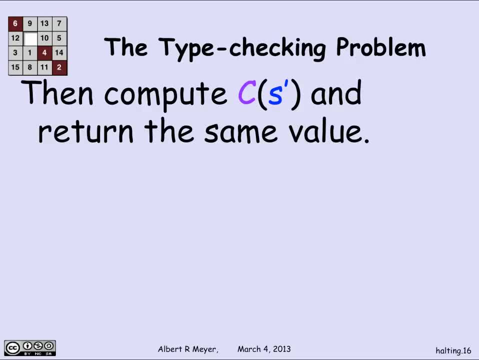 So the way H works: is given input S, it constructs the program S prime and applies the type checker C to S prime and returns the same value that C does. So what we can figure out by these definitions is that S halts the string. S is a halting string. 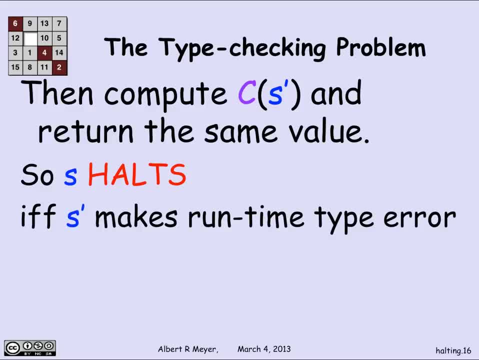 if, and only if, the string S prime makes a runtime type error, Because remember the interpreter, which is what S prime was behaving like, was watching what S simulating, what S did And if S was going to halt successfully, S prime makes a runtime type error. 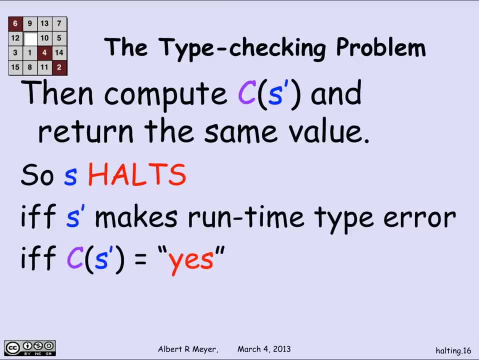 That means that C is going to say yes to S prime. Yes, it has a runtime type error And, by definition of H, that means that H of S says yes because H of S constructed S prime and fed it to C. On the other hand, if S does not halt, 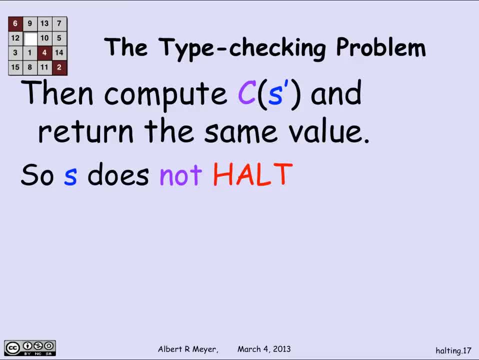 that means that something else goes wrong with S. It's not going to successfully return. Then S prime, when it's simulating S, is never going to make a runtime type error because that's the way S prime goes, Whenever it detects that there would. 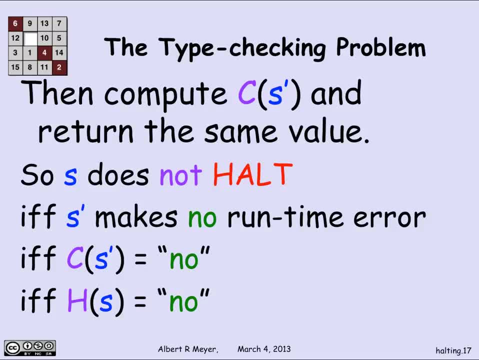 be about to be a runtime type error. it skips it. So S prime is likely to keep running forever because it's simulating this program S that doesn't halt but it won't make a type error And that means that C of S prime is going to say no, no type. 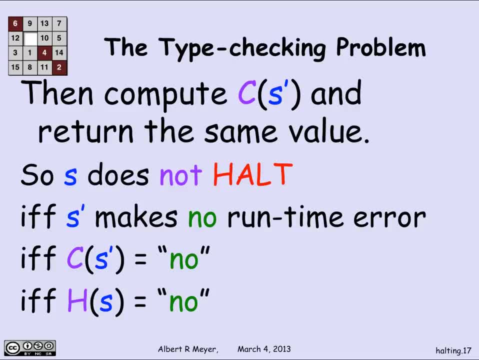 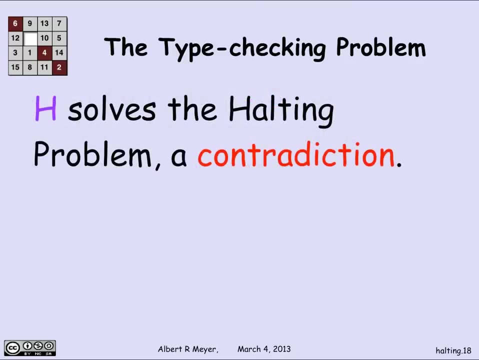 error and H of S is going to say no And that means that when S does not halt, H of S properly says no. In other words, I've just walked through the argument that this procedure H that I've described actually is a decider for halts. 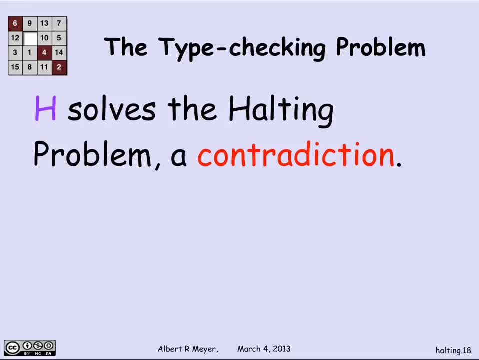 And that's a contradiction. The H that I gave you would solve the halting problem if there was a perfect type checker. And there can't be a halting problem, decider so there can't be a perfect type checker C must make a mistake. 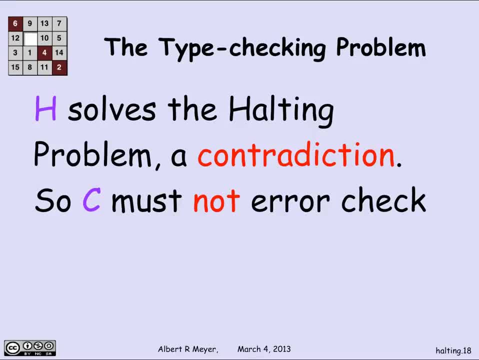 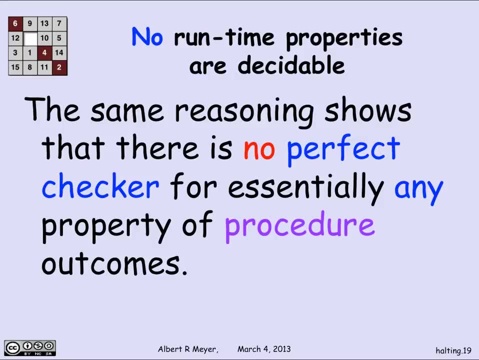 It can't accurately predict runtime errors, And that is an example of how you reason from this kind of contrived halting problem. that's sort of self-referential whether the string procedure applied to its own definition halts or not, And we can apply it to all sorts of questions and properties. 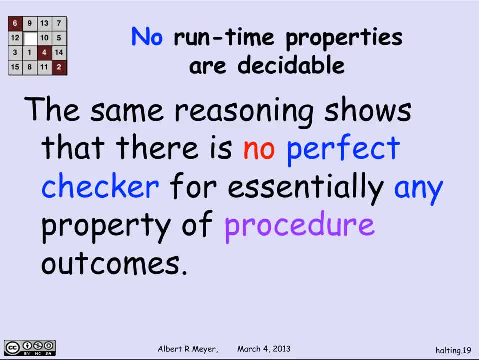 of procedures that we really care about And in fact the same reasoning really shows that it's not just type checking. That's a kind of arbitrary example, But there's more or less no perfect checker for any kind of property that procedure outcomes might. 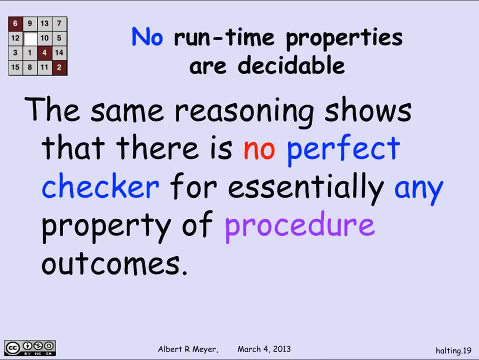 exhibit, which is why a theoretical computer scientist interested in the theory of computation have great respect and interest in diagonal arguments, because they crystallize a whole set of absolutely logical intrinsic limitations on the power of computation.